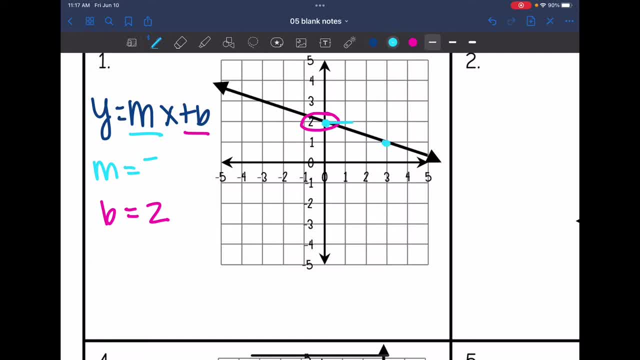 And I'm going to draw a slope triangle and find the rise, which is 1,, over the run, which is 3.. So my slope is negative 1- 3rd. So my equation in slope intercept form would be: y equals negative 1- 3rd, x plus 2.. 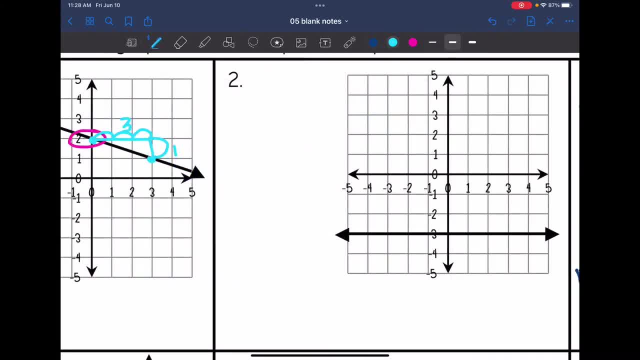 All right, let's go ahead and draw a slope triangle. Let's look at number 2.. So we have one of our special cases. We have a horizontal line, So that means that the slope is 0. And then our y-intercept is negative 3.. So if I were to write this in slope: 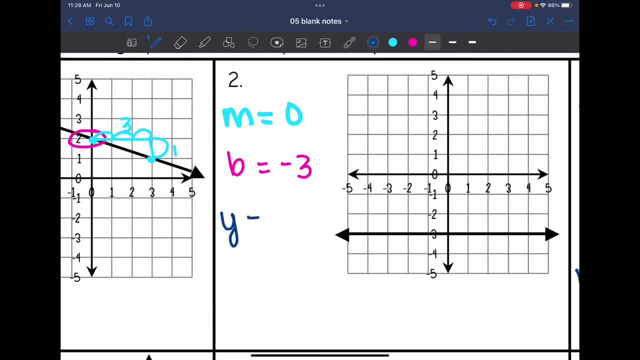 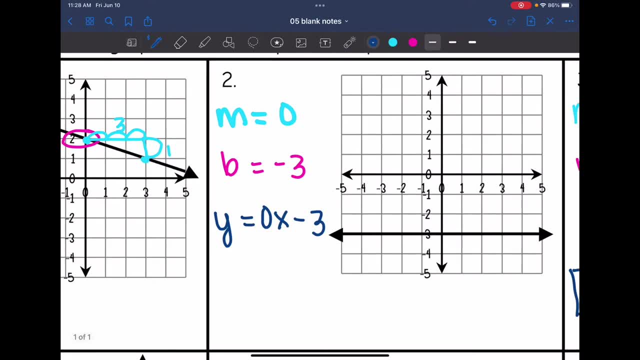 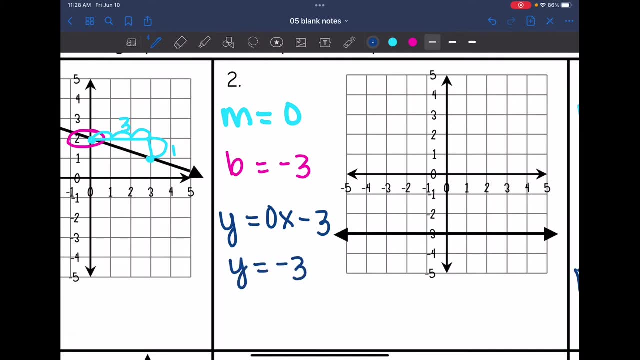 intercept form, it would be y equals 0x minus 3.. This 0x is unnecessary. If we have no x's, we don't need to write anything down. So it would just be y equals negative 3. for our final equation, If you think back to our acronym from the beginning, 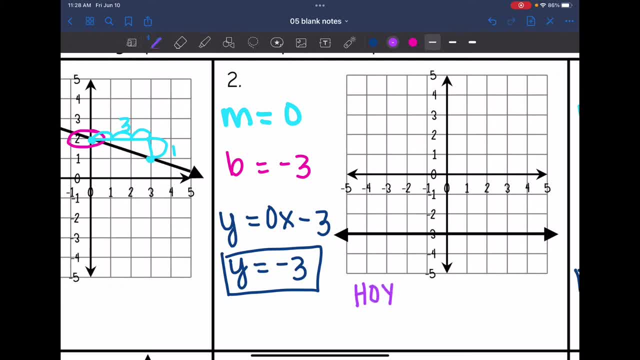 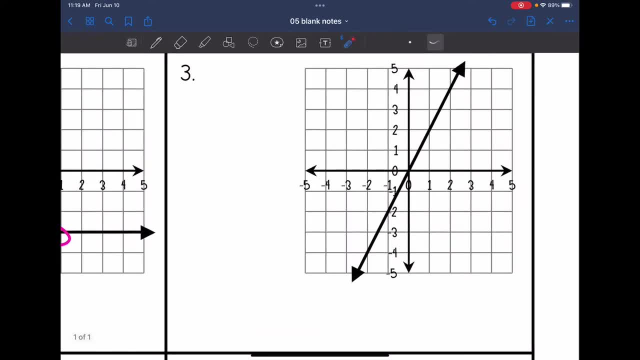 Hoi Vux. this is the Hoi part. This was a horizontal line with a 0 slope, So that's how we knew it had a y equals equation. All right, let's look at number 3.. I have a positive line, So 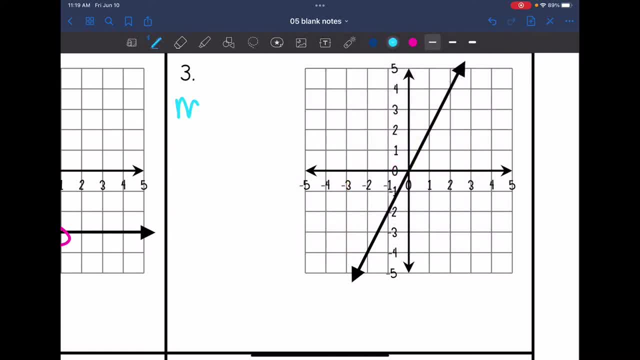 I'm going to write it in: y equals mx plus b form. I need the slope and I'll need the y-intercept. The y-intercept is 0.. Since this line is crossing through the origin. And now let's find the slope by drawing a slope. 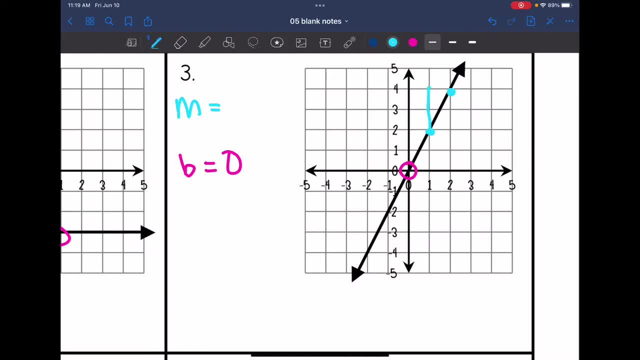 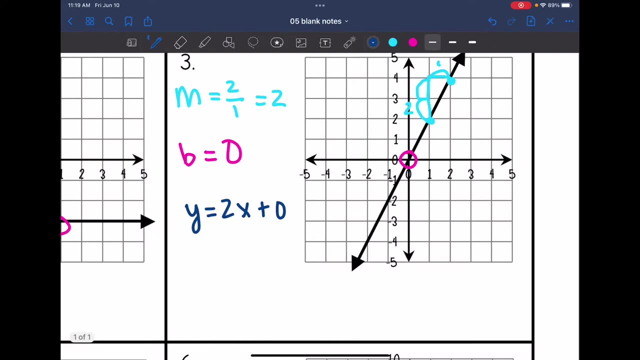 triangle with two perfect points. My rise is 2.. The run is 1. So the slope is 2 over 1 or 2.. So my equation is: y equals 2x plus 0.. We can simplify that because this plus 0 is kind of. 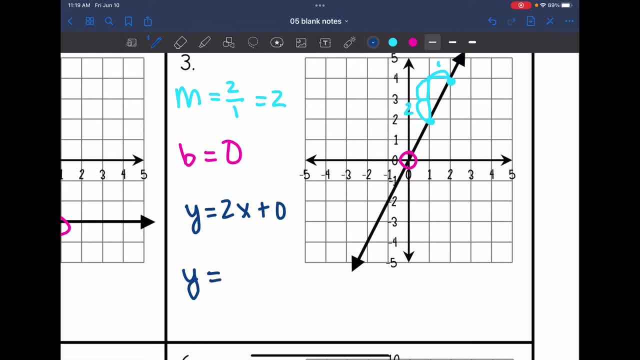 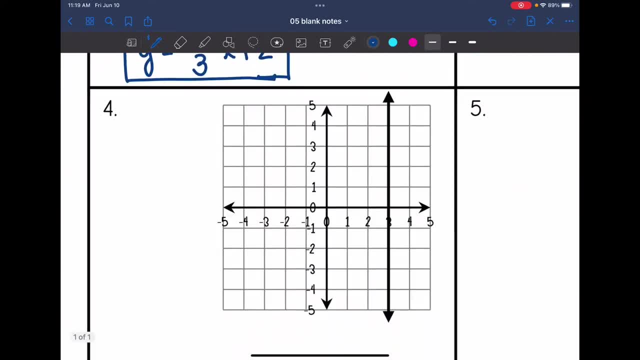 unnecessary, So it'll just be: y equals 2x. All right, let's look at 4.. So I have a vertical line, So it's going to be one of our special cases. The slope is undefined And the y-intercept is none. It is never going to intersect the y-axis. 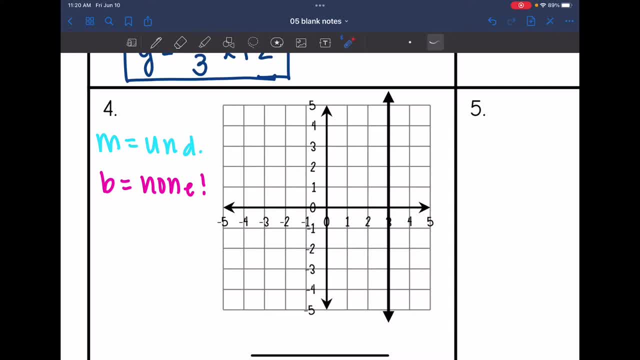 since it's parallel with the y-axis. So that kind of tells us that this is going to be a different equation. So this is going to be an x, And this is going to be an y, And this is going to be an x. 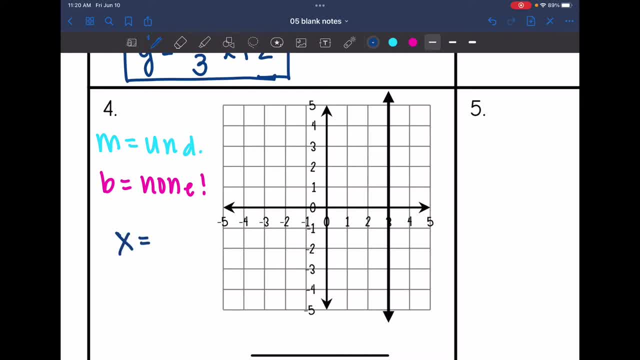 So this is going to be an x And this is going to be an x And this is going to be an x. And this is equals equation because it's going through the x-axis And all of the x values of this equation are always going to be x equals 3.. If you think about our acronym from the beginning, 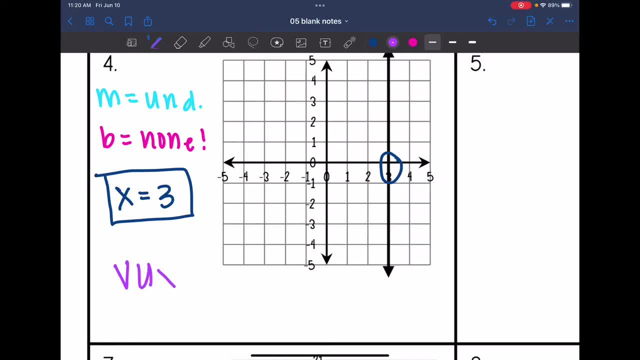 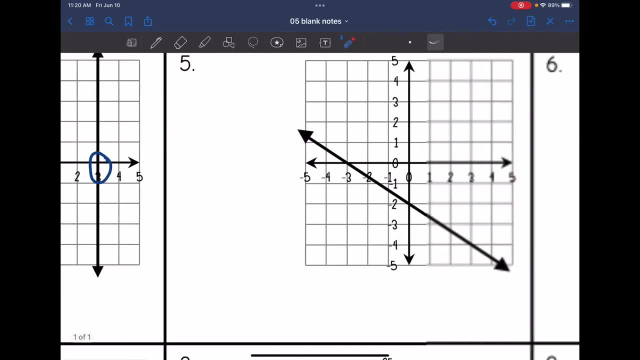 this is the VUX part. in Hoi VUX, We have a vertical line with an undefined slope, So it's going to have an x equals equation. All right, number 5, I have a negative line, So I'll need the slope. 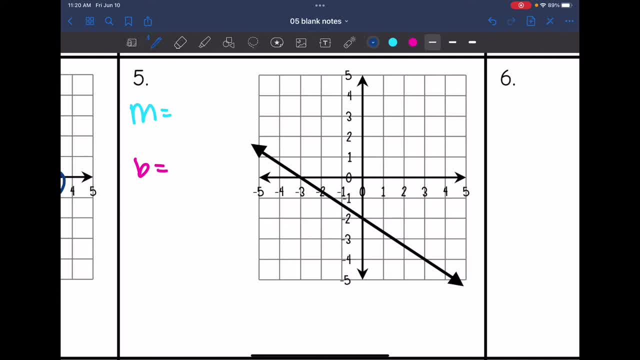 And the y-intercept, And then I can write it in slope-intercept form. So let's start with the y-intercept. This graph is crossing the y-axis at negative 2.. And then my slope. I'm going to find two perfect points. Draw my slope triangle. The rise is 2.. The run is 3.. So the slope is negative. 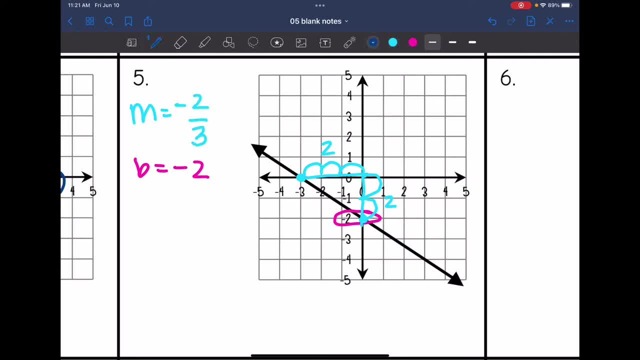 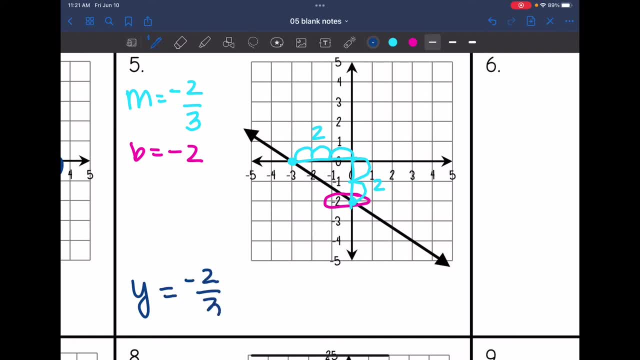 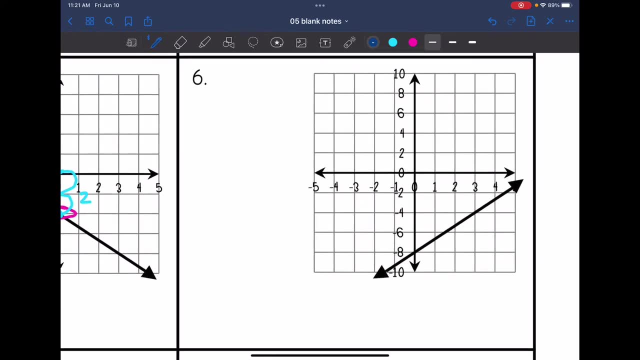 two-thirds, Don't forget the negative. So my equation and slope-intercept form are going to be: y equals negative two-thirds, x minus 2.. All right, number 6,. I have another positive slope, So I'm going to need the slope and the 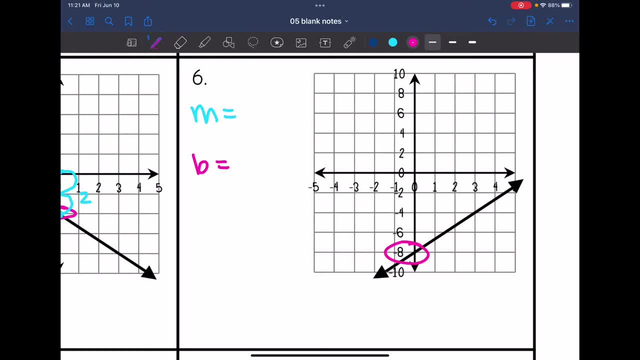 y-intercept. The y-intercept is negative, 8. And then my slope is positive. I need to be careful with counting the rise, because my y-axis is counting the rise. So I'm going to need the slope and the y-intercept, So I'm going to draw my two perfect points. My rise is two spaces. 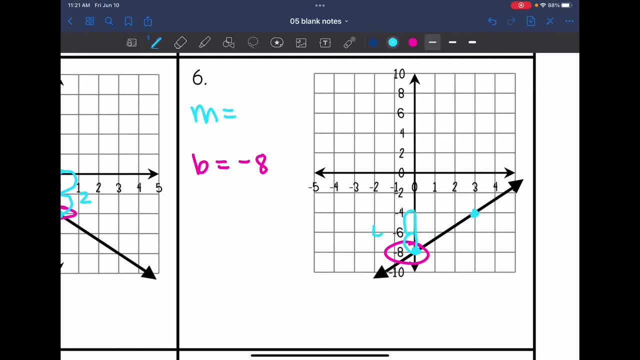 but I have to count that by two, So it's really 2, 4.. And then the run is 1,, 2,, 3.. So my slope is four-thirds. So now I have the slope and the y-intercept, So I can write it in slope-intercept. 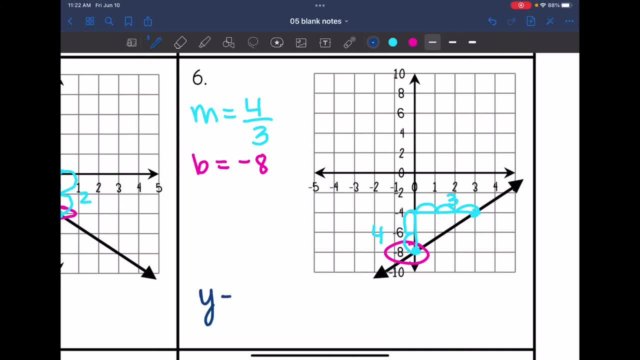 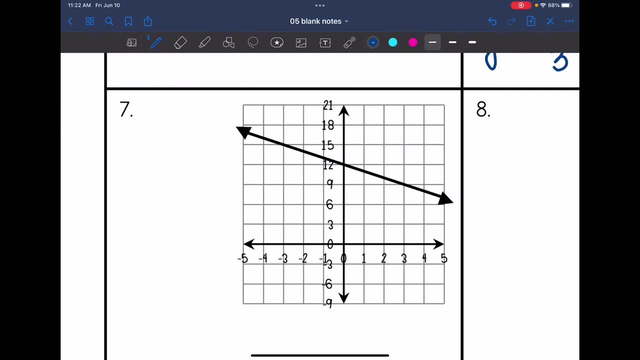 form It'll be: y equals four-thirds x. All right, number 7,. I need the slope and the y-intercept to be able to write this equation. y-intercept is at 12. And then I see that my slope is negative, So I'm going to go ahead and put that. 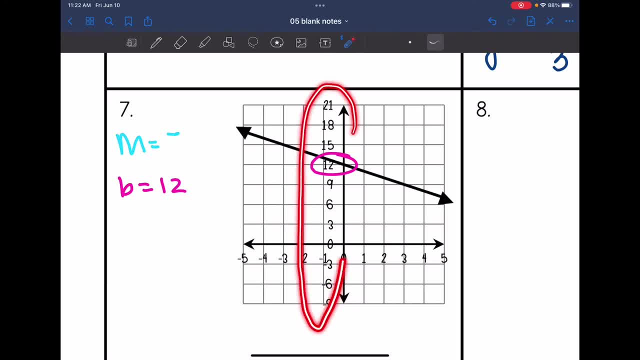 And before I count the slope, I'm going to recognize that the y-axis is counting by three, So I'll have to count my rise by threes. So here's my two perfect points. Let's draw our slope triangle. The rise is 3.. And the run is also 1,, 2,, 3.. So my slope is. 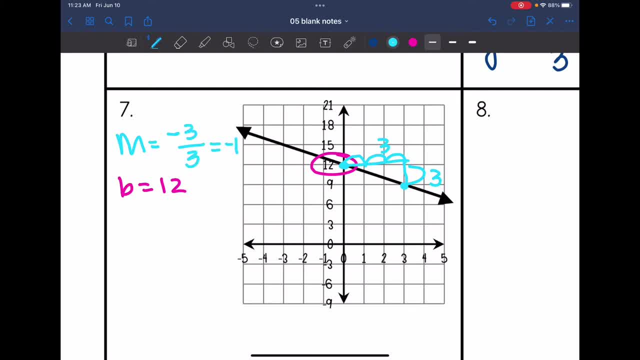 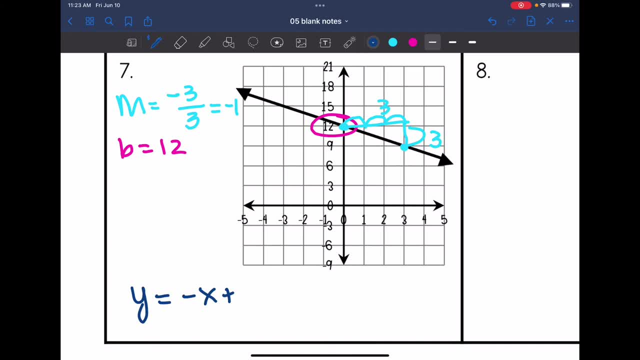 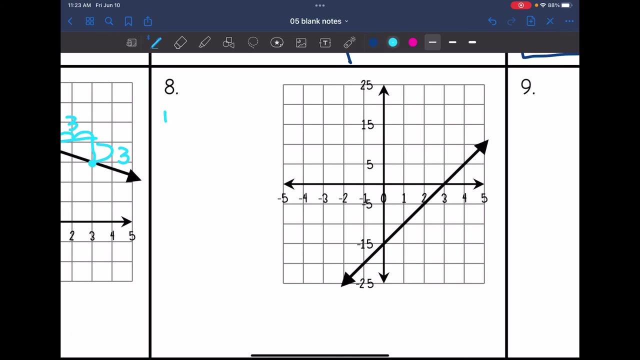 negative 3 over 3, which simplifies to negative 1.. So the equation would be: y equals negative x plus 12.. You could put that one there, but it's a little more proper to just leave it as negative x. Okay, number 8.. I need the slope And I need the y-intercept. y-intercept is negative 15.. 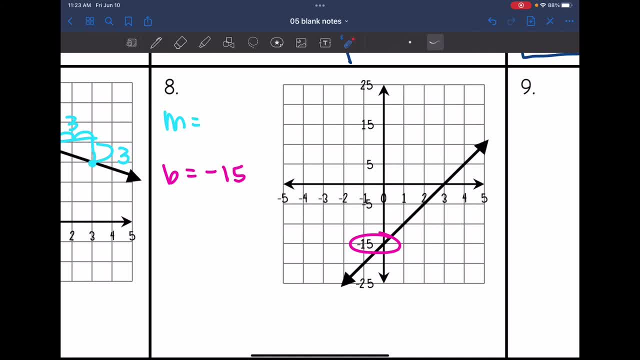 And the slope is positive. Let's be careful when we're counting the rise. It looks like we're counting by fives. That'd be 5, 10, 15.. Yes, we're counting by fives, So there's a perfect point. There's a perfect point. My rise is one space, but that's really. 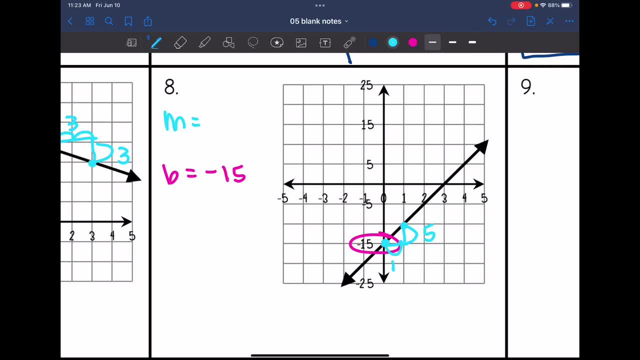 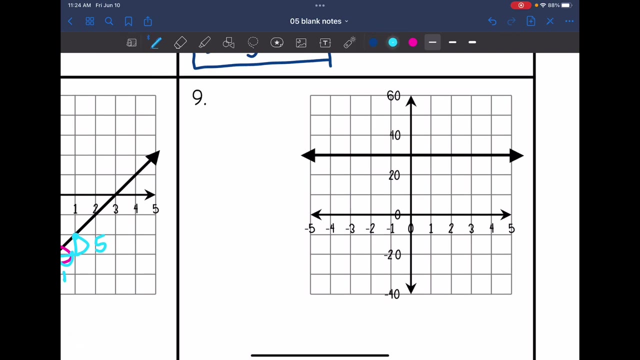 five, And then the run is still just counting. So the slope is 5 over 1, which simplifies to 5.. So our equation in slope-intercept form is: y equals 5x minus 15.. And number 9.. I have a horizontal line. My slope is 0.. 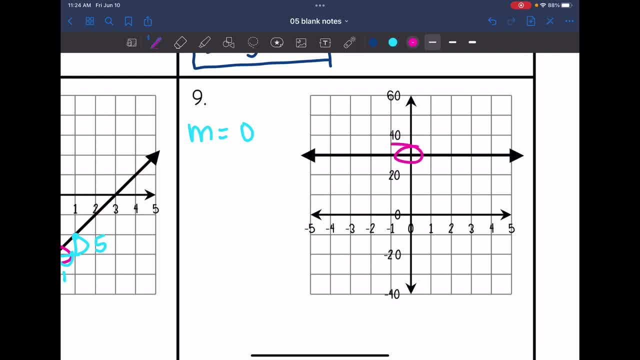 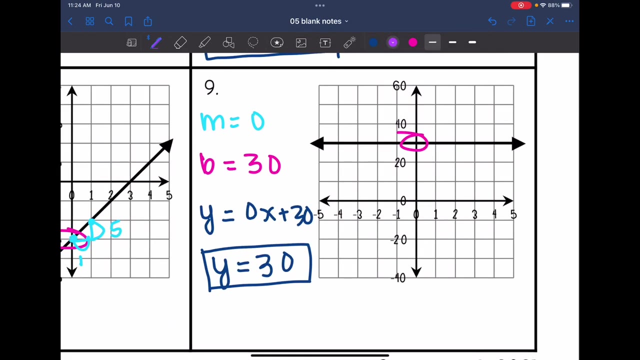 And my y-intercept is between 20 and 40. So that is 30. So my equation would be: y equals 0x plus 30, which simplifies to y equals 30.. And if you think about our acronym for our special cases, this would be the Hoy and Hoy Vux. 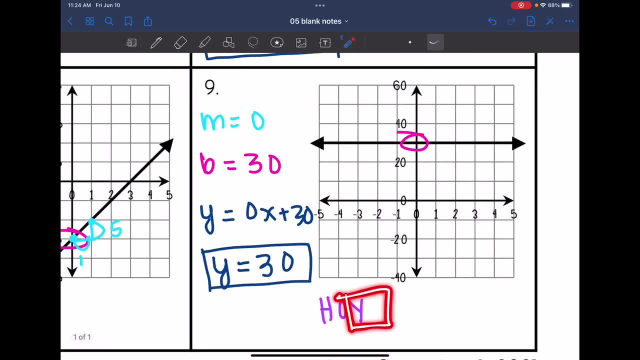 We have a horizontal line with a zero slope and a y equals equation.